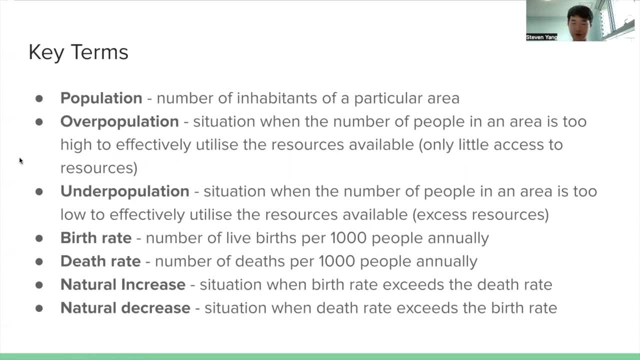 And underpopulation is the direct opposit of overpopulation, and so this is: you are the direct opposite of overpopulation. so this is your situation: when the number of people in an area is too low. so effectively utilize the resources available. so the resources are in excess that are not everyone in the population can actually utilize those, all of those limited resources effectively. 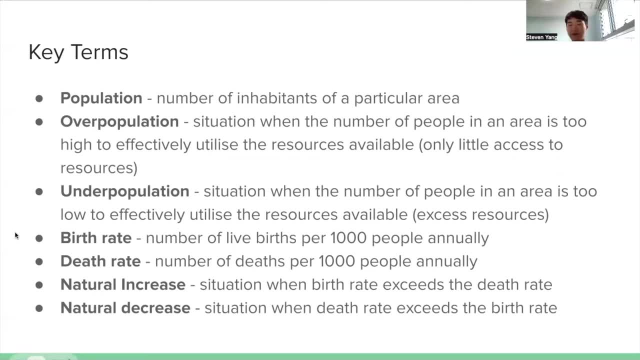 And birth rate is the number of live birth per 1000 people annually, and death rate is of course, the opposite. So Bennett is underneath 2%. So it's the number of deaths per 1,000 people annually, And natural increase is the situation. 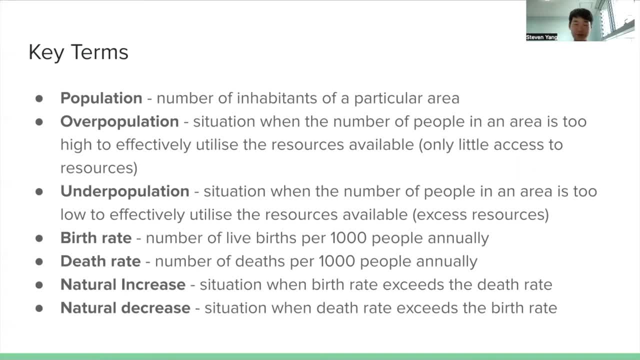 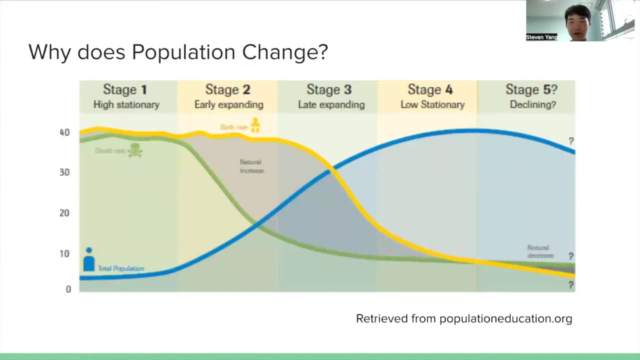 when the birth rate exceeds the death rate, And natural decrease is, of course, the situation when it's vice versa, So when the death rate exceeds the birth rate. So why does population change? So what you're seeing here is a demographic transition model. 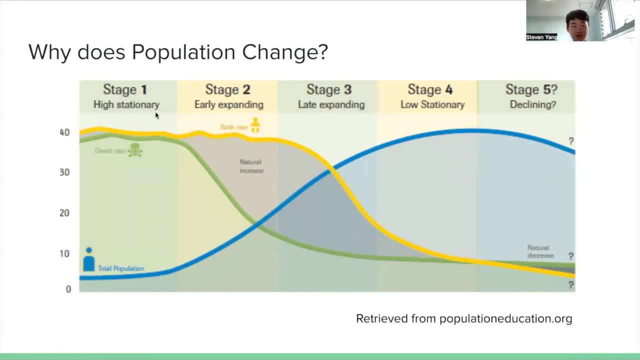 which relates a country's population change based on the change in economic status. So if you follow my cursor, you can see three lines. So we have a yellow line, which is the birth rate, And we have the green line which is the death rate. 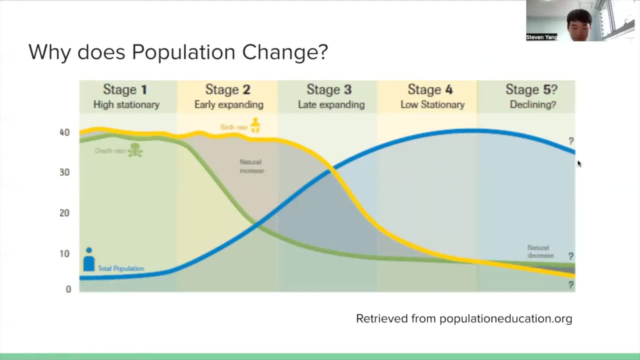 And we have the blue line, which is the total population. And to start off with stage one, here is the high stationary period, when the country's economy is not developed yet. So therefore the death rate is very high due to the high infant mortality rate. 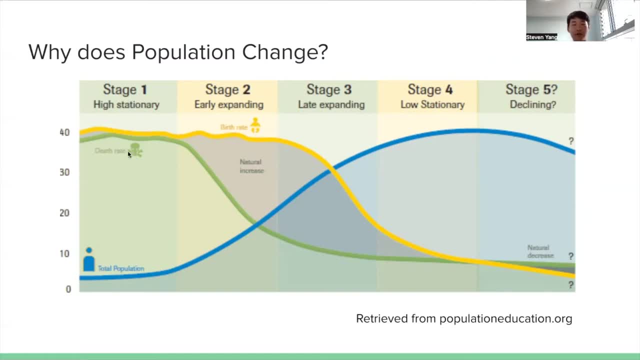 and the lack of advance in medical technology. So here you have households having many children, but also many deaths with a very low life expectancy. So since the birth rate and the death rate are equal, you have a stationary population. And when we move on to stage two, 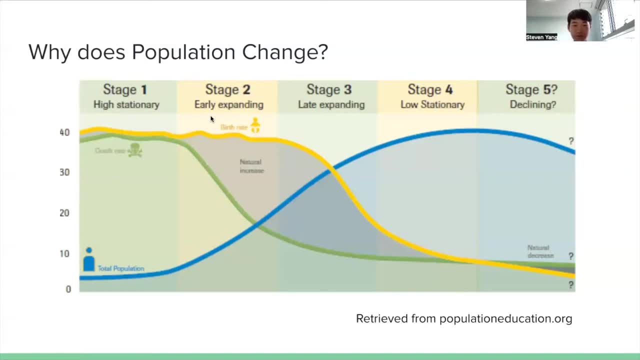 this is the early expanding period when the death rate decreases as there are advancements in medical technology, as the country starts to develop, which decreases the infant mortality rate and increases life expectancy. But still, of course, change doesn't happen rapidly. So here we still have the birth rate constant. 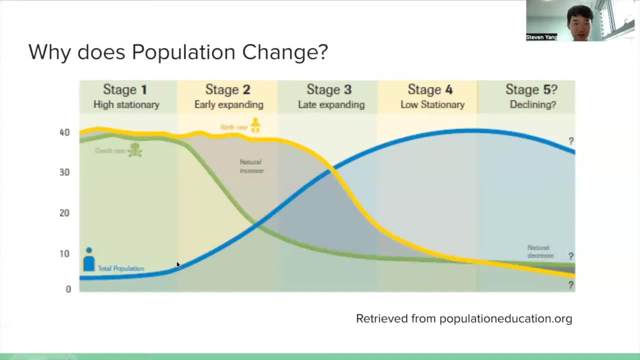 and a high rate. So this you can see: the total population starting to grow here And in stage three. this is the late expanding period, when the birth rate starts to decrease as there's emancipation of women and the cost of living increases, since the economy has been developed significantly. 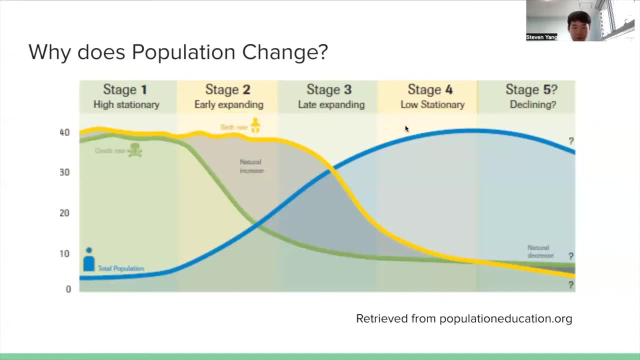 And stage four is the low stationary period, when the birth rate and death rate are equal, but this time they are all low And because of that the population growth starts to curve and starts to become in a stationary position. but the population is much higher than that is in stage one. 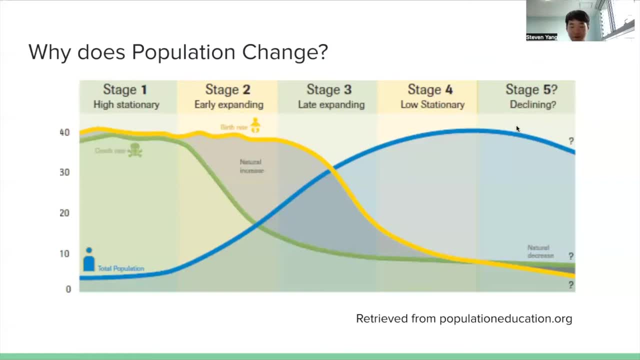 And in stage one, I'm sorry, in stage two, I'm sorry in stage three, stage four, stage five is the declining period, when the population starts to decline as the birth rate is lower than the death rate. So the demographic transition model gives you an overview. 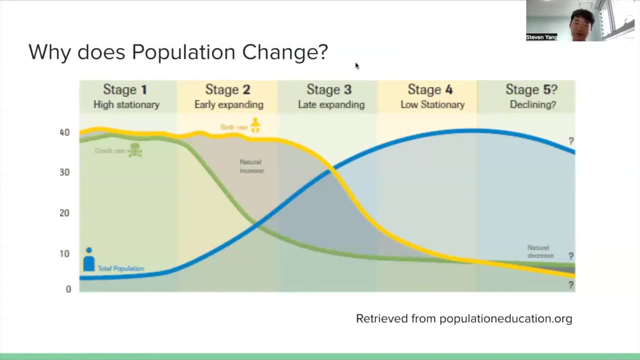 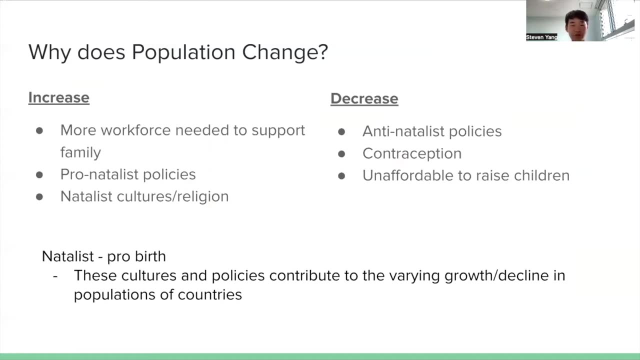 how the population changes as a country develops economically, And here are some other factors that stimulate population change- And many households in less economically developed nations want more children as a workforce to support them. So, of course, there's a lot of work to be done. 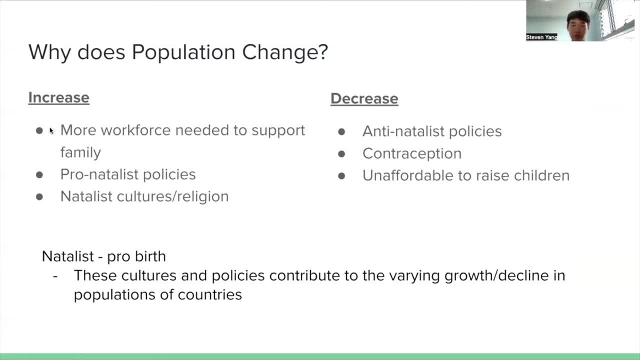 Of course, households have many babies to actually support their family, And also there are pro-natalist policies. so which is basically pro-birth in nations that need a growing population, And some cultures and religion are also pro-natalists too. 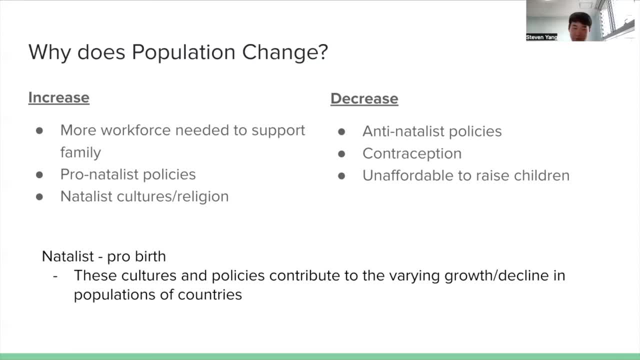 which opposes contraception and considers birth as a blessing, And contraception is the method to actually inhibit pregnancy. And for the factors that actually decrease population growth or actually creates a population decline are anti-natalist policies. So one of the anti-natalist policies 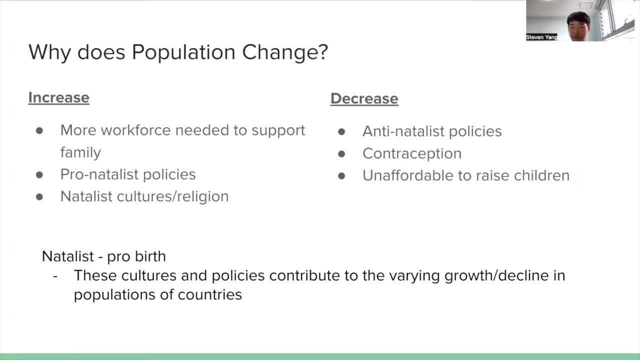 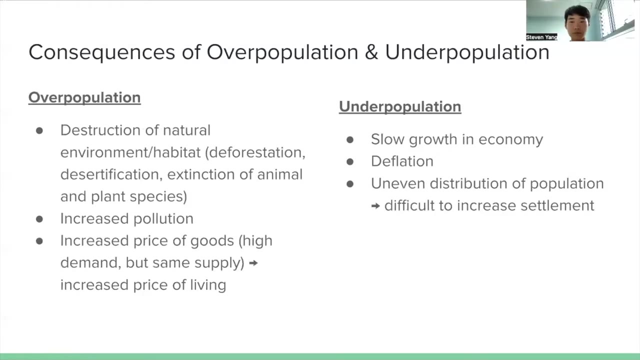 is the Chinese one-child policy, which I will talk about later, And of course, there are the use of contraceptive methods and also being unaffordable to raise children. This actually pertains to the more economically developed countries And I would like to talk about the consequences. 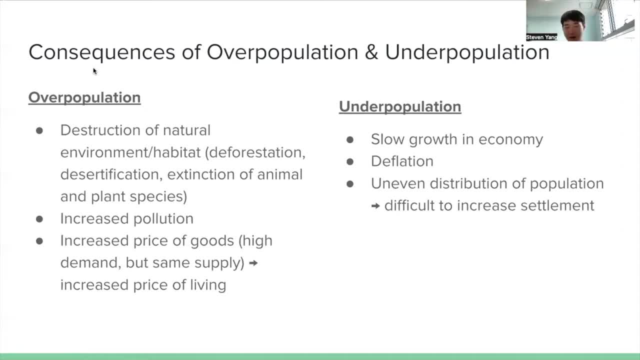 of overpopulation and underpopulation because of course, both having too high of a population or too low of a population have repercussions. So the consequences of overpopulation includes the destruction of the natural environment and habitat of wildlife, along with increased pollution. Also, the price of goods will increase. 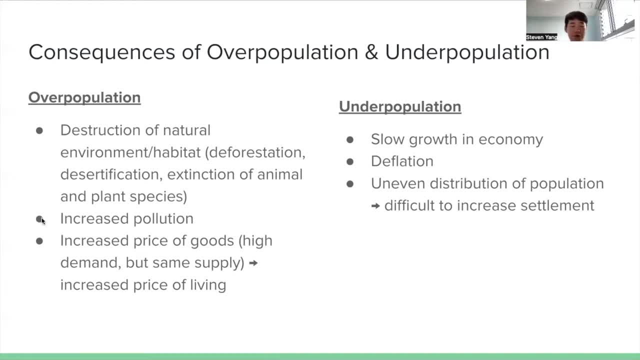 since there's increased demand for the same supply, though, which then leads to the increased price of living. Of course, not all people are going to be able to afford the high price of living, So this is going to be a social problem And the consequences of underpopulation. 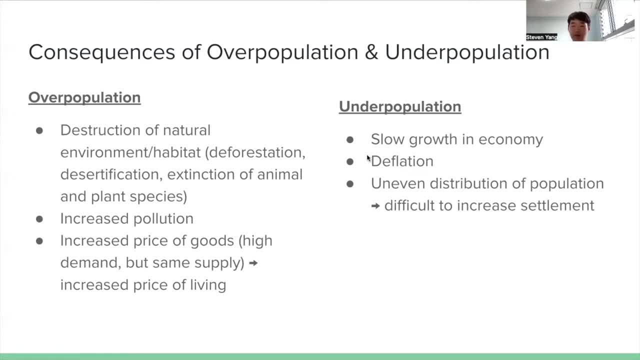 include a lack of growth in economy and also deflation and the uneven distribution of population that creates difficulty in increasing areas for settlement. So let's say you might have an area that you want to live in but unfortunately nothing has developed there, so you just live in like just the middle of nowhere. 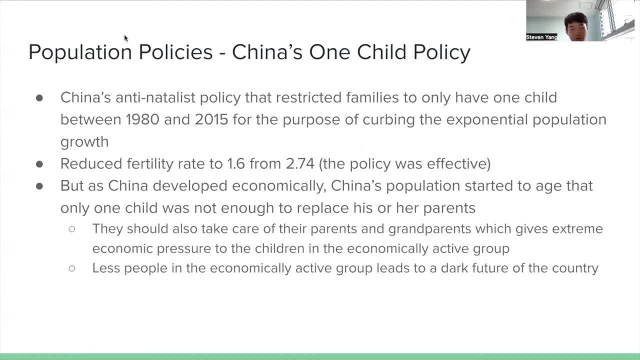 so one example of a population policy is china's one child policy. so it is a. it was an anti-natalist policy which restricted families to only have one child between 1980 and 2015 for the purpose of curbing the exponential population growth. and well, it did reduce the fertility rate to. 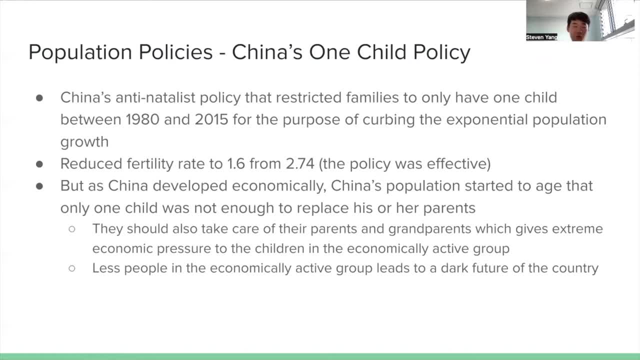 1.6 from 2.74 per couple. well, yeah, then it proved that the policy was effective. but china's population started to age, as i mentioned in the demographic transition model. so, as china has economically developed, the life expectancy has increased, but the fertility rate. 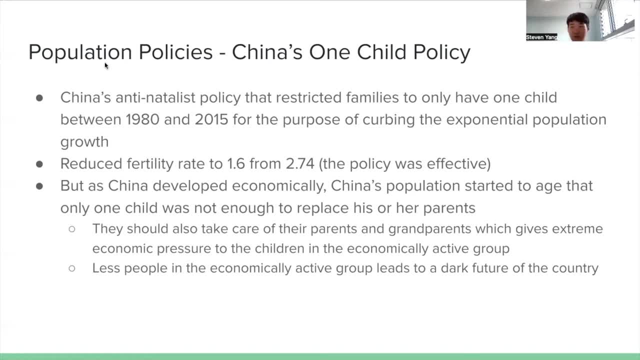 has decreased. so, you, you, we could say that china, uh, is currently in stage four and is at a risk to actually go into stage five, which which creates a natural decrease. and the problem here is that the number of people in economically active group, which i will talk about in some other population topics, uh, they will be. 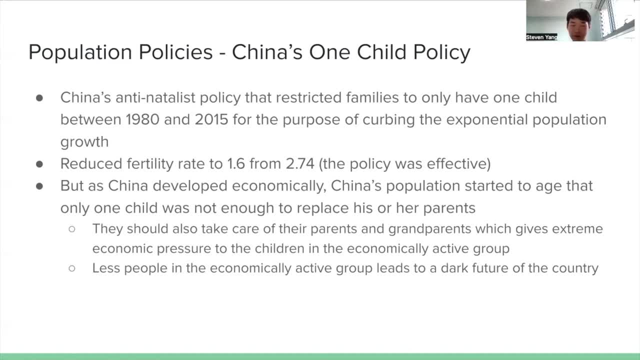 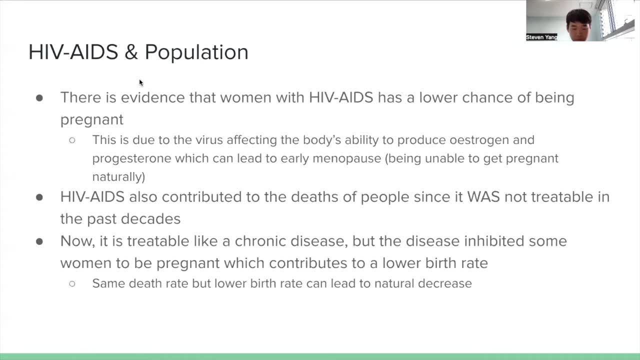 decreased, but they will have to take care of their parents and elders, so this decline can also lead to the dark future of the country. you and another factor that affects population is, uh, hiv aids. so hiv is a human immunodeficiency virus. so this virus affects the ability of women to produce estrogen or progesterone. oh well, of course. 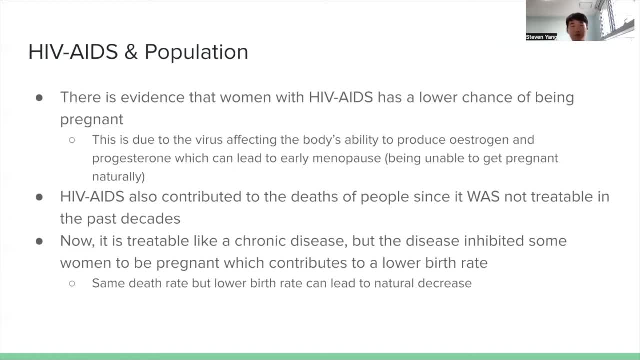 hiv and aids. well, they usually uh produce the. the main problem of hiv and aids is that they literally make the immune system to malfunction and they're not able to produce estrogen or progesterone. so they're not able to produce estrogen or progesterone. 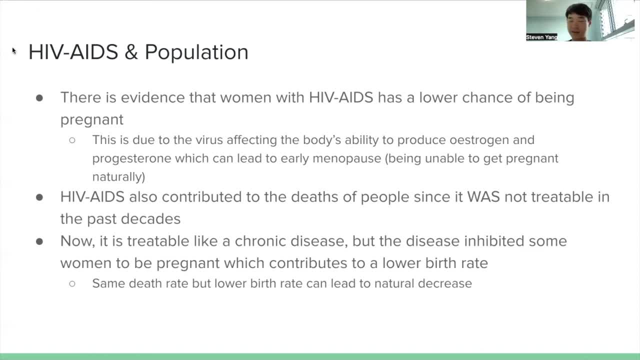 which, um, in the past, just literally was a signal, was a death with a death penalty for patients who actually have that there was no way to cure. but in this context, um, this could lead to early menopause, which is the state of being unable to become pregnant naturally and, yes, of course, in the past, 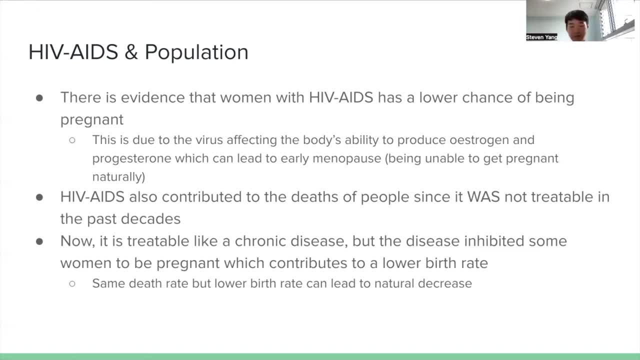 um this. ain't this contribute to the increasing of death rates? but in the present day this virus could be treated as a chronic disease, like diabetes and other diseases, like diabetes and other diseases or high blood pressure. but still inhibiting women to be pregnant contributes to a lower death rate. 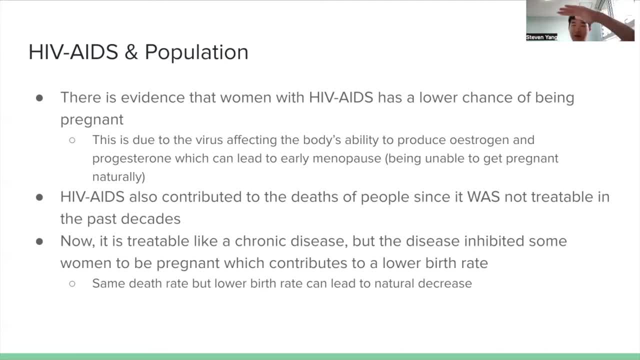 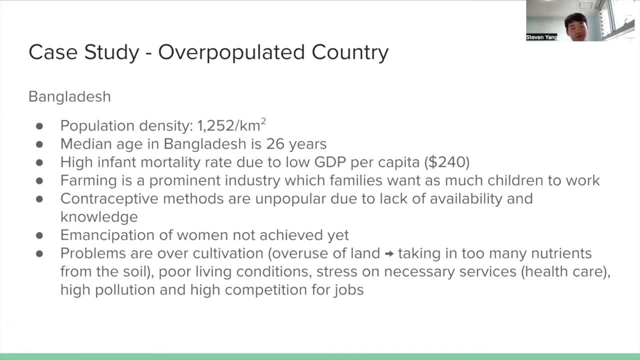 now, which could lead to a natural decrease. so you have the same death rate, but the birth rate is lower. that's why the country will move into a natural decrease. and now i'll introduce you to the case studies. the first case study is for an overpopulated. 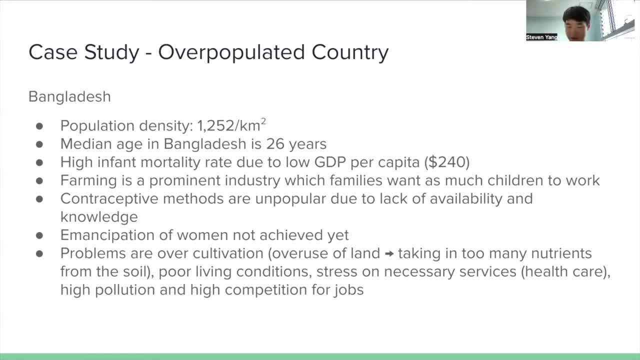 country, which is bangladesh, and as an introduction, with place specific detail which is very crucial in your seven more questions. bangladesh has a population density of 1 252 people per square kilometers and the median age is 26, which is very young. the reason why bangladesh is overpopulated. 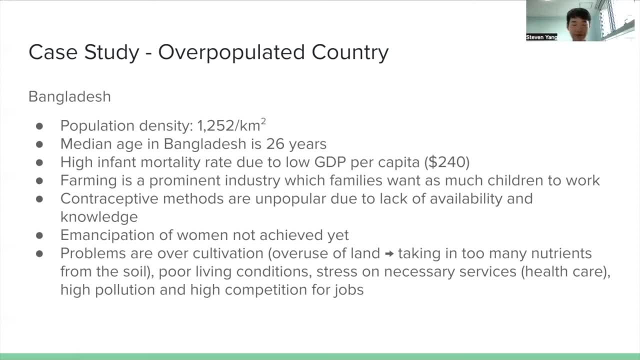 so this is because the infant mortality rate is very high due to a bad economy, with low gdp per capita of 240 dollars only, which leads to high birth rate because families want more work, work force and farms, with contraceptive methods being unpopular too due to the lack of ability. 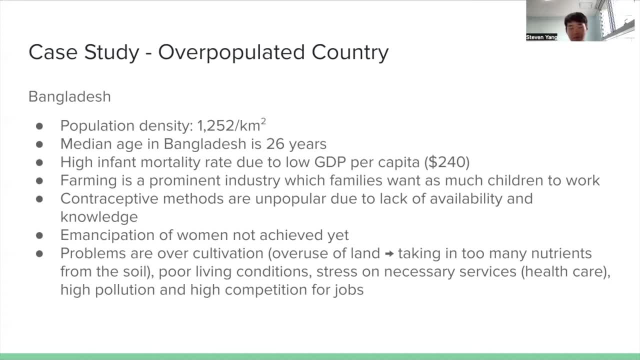 and knowledge, along with the emancipation of women, not achieved yet. so we could say that bangladesh is still in uh stages two, which uh we stage of one and two, where you have the high birth rate and the manageable of women, has not been achieved yet. and the problems of ee a, of overpopulation, can be overcome and are predominantly of men since the early 20s, but social care- aging theалось can also causeれた demands, while developing a Expert's focus on mental prepared for special care. 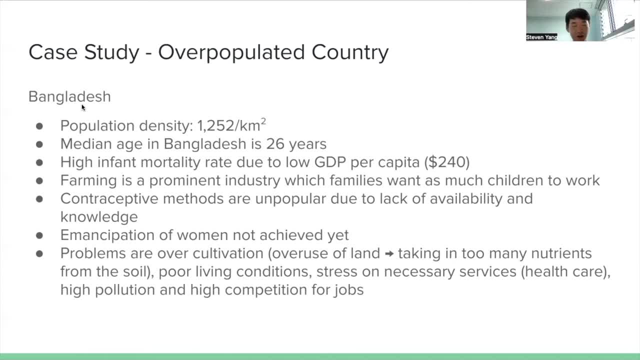 And the problems of this overpopulation can be over cultivation in the rural areas, which is the overuse of farmlands that leads to taking in too many nutrients from the soil, then the soil would lose its fertility, And in urban areas especially. 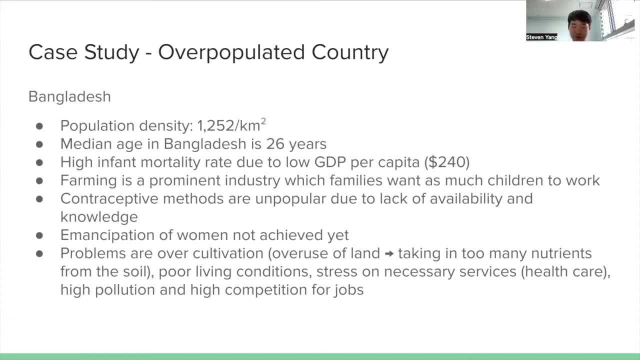 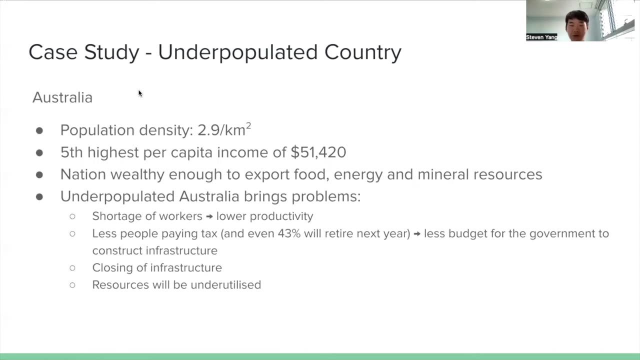 you would have poor living conditions, stress on necessary services, especially in the healthcare, and high population and competition of jobs, which leads to high unemployment, which leads to poor living conditions and competition of jobs. And my second case study that I'd like to introduce to you: 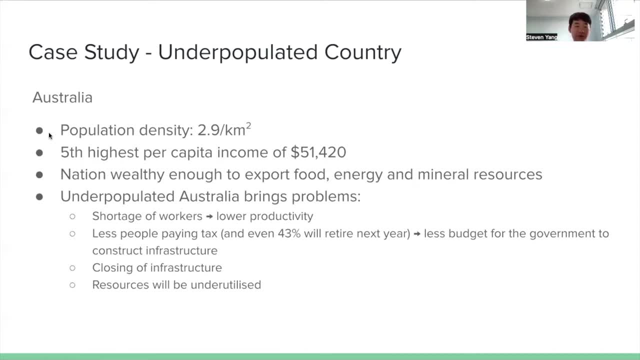 is for an underpopulated country which I chose, Australia. So the population density is only 2.9 square kilometers of people per square kilometers, compared to the 1,252 people per square kilometers in Bangladesh, And the Australia's economy is really good actually. 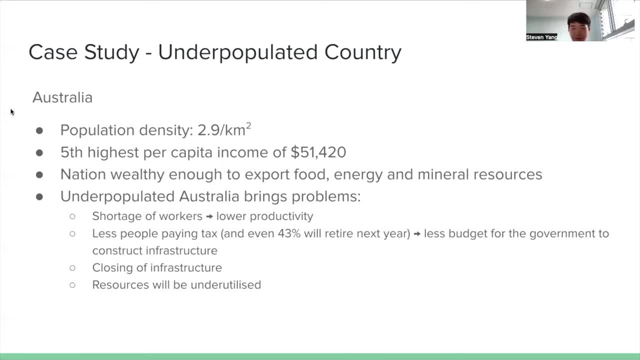 So it has five. it's ranked in the fifth highest per capita income of 51,000, and the US economy is number one with $7,420, and along with high exports, leading to a higher standard of living, which would bring the nation to an under populated state. 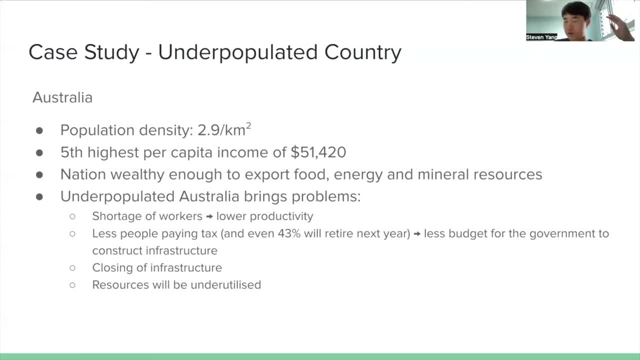 So, since there's a high standard of living, because the living also increases, where less families will be actually be affordable to raise children, And the problems of this underpopulation can be some shortage of workers leading to a lower productivity in the economy. So there are problems. 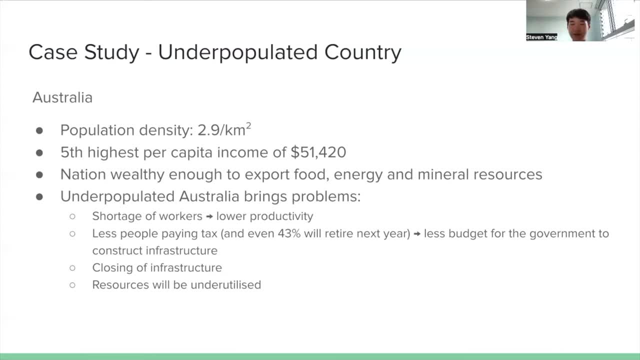 So the problems of underpopulation can be some shortage of workers leading to a lower productivity in the economy. So there are problems of underpopulation. there is no guarantee that australia would actually maintain their strong economy along with their fifth highest per capita income in the future. and we have- we're going to have less people. 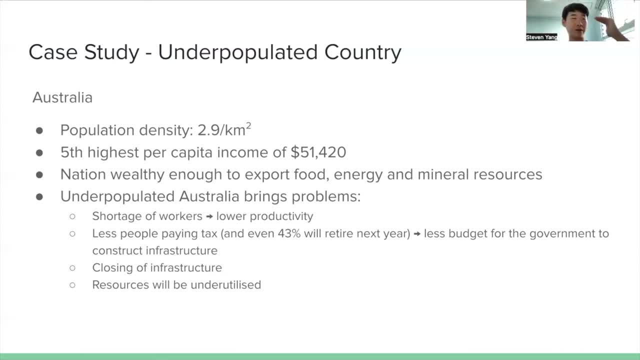 paying tax as the birth rate decreases, but people in the elderly ranges will increase and also we will have closings of infrastructures and the underutilization of resources. so even though you have those great, marvelous, magnificent natural resources, well, the country won't be able to use it because of the underpopulation, so that's why the economy is going to shrink. 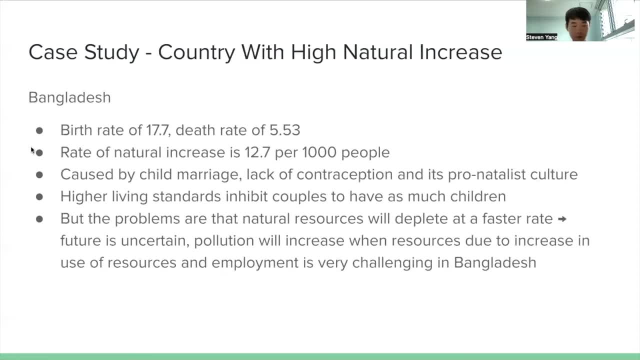 the next case study is for a country with a high natural increase. so i chose bangladesh again, since it has a really really high birth rate of 17.7 and a death rate of 5.5 per 1000 people, and you could realize that the difference is very. 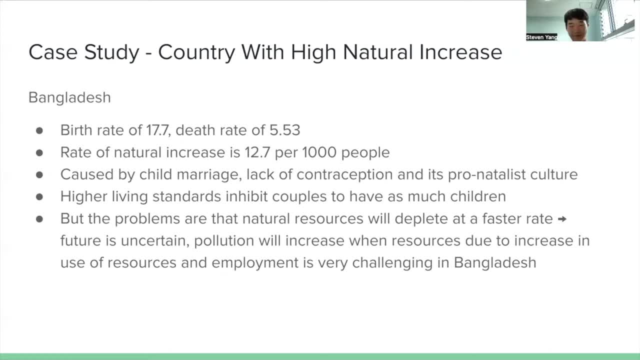 significant- 17.7 versus 5.53- and the rate of natural increases- 12.7 per 1000 people- which is caused by child marriage, lack of contraception and the pro-natalist culture, and also the higher living standards, will inhibit couples from having many children too, and the problems coming from a 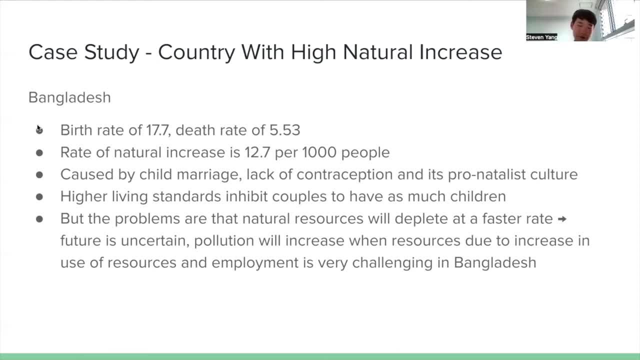 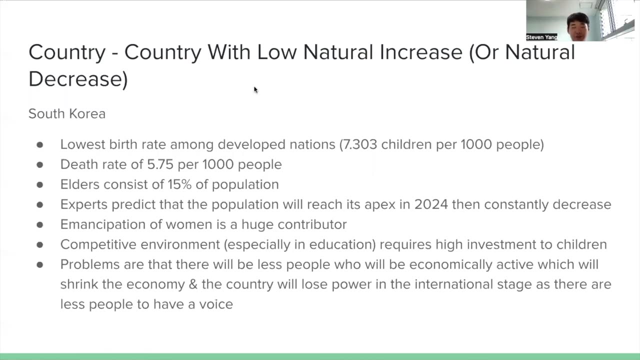 high natural increase is very similar to the problems of overpopulation, so there will be an uncertain future. there will be an increase in pollution and, of course, high competition for employment. and the last case study i'll be talking about is for a country with a very low natural increase. 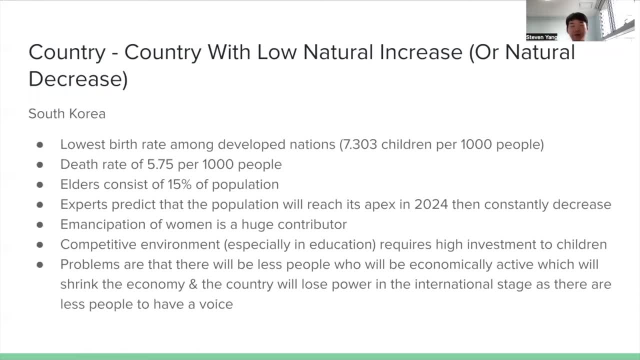 or i mean actually we could call this a natural decrease. so south korea is a prime example of this. so this country has the lowest birth rate among developed nations, with only 7.303 children per 1000 people, but the birth rate of children is very low and the birth rate of children is very low. 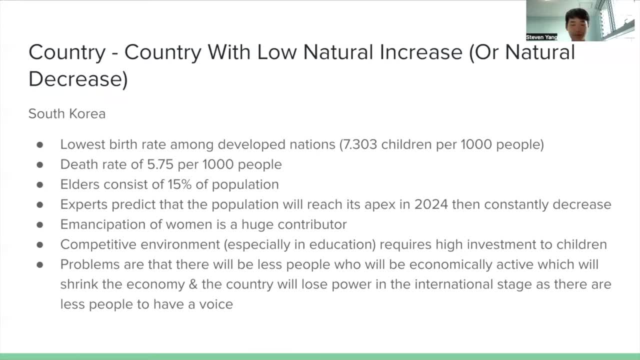 it has a death rate of 5.75 per 1000 people. well, of course, the difference between the birth rate and death rate is much closer than we than when we compare it to bangladesh, and elders consist of 15 percent of the population, so that makes experts predict that the population will reach its apex in. 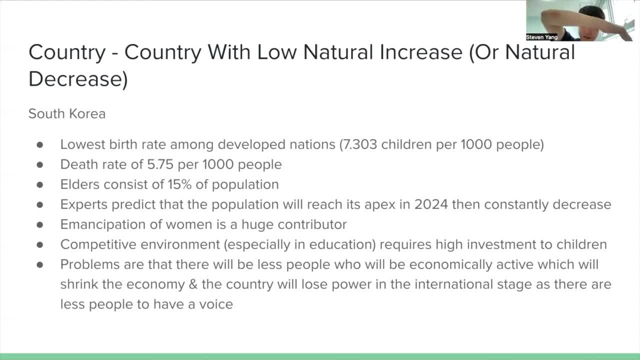 2024, and then the population will constantly decrease and the emancipation of women in the country is also very low and the birth rate of children is very low. and the birth rate of children is also a very, very huge contributor, along with the competitiveness of the society and, of course, 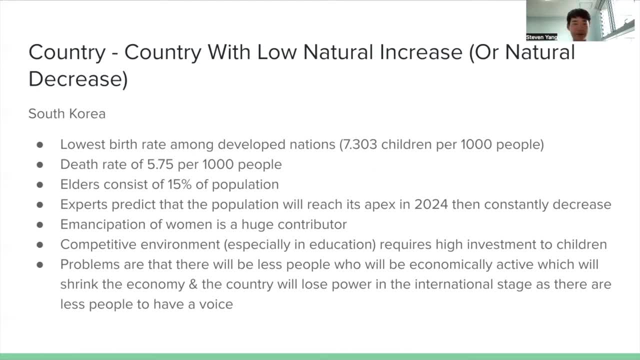 many of you will know that south korea is very, very competitive in education, which requires high investment in organizing in private institutes called hagwons that is. that can be hard to afford for some families. so the consequences of this is that the economy will shrink due to having less. 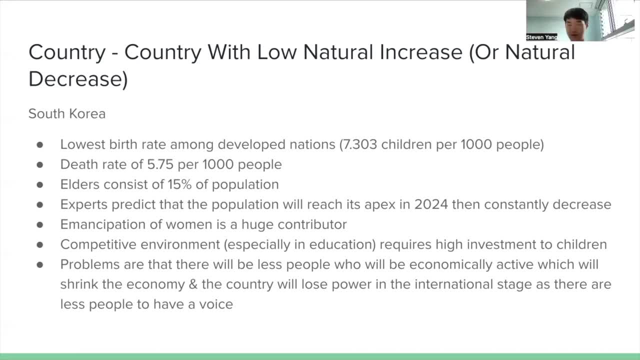 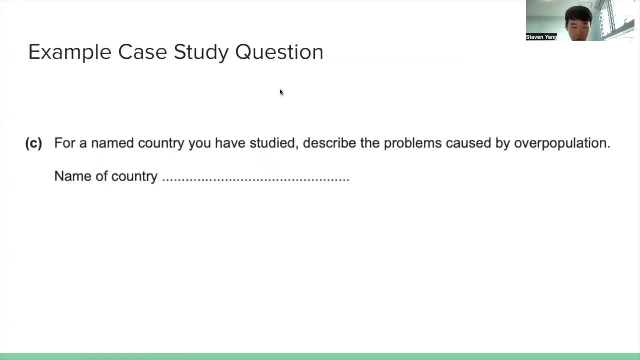 workforce, along with losing power in the international stage as there are less resources to represent in those international organizations. so since we covered all these case studies required for topic 1.1, i will introduce a seven mark case study question for you guys. so the question is for a named country you have studied. describe. 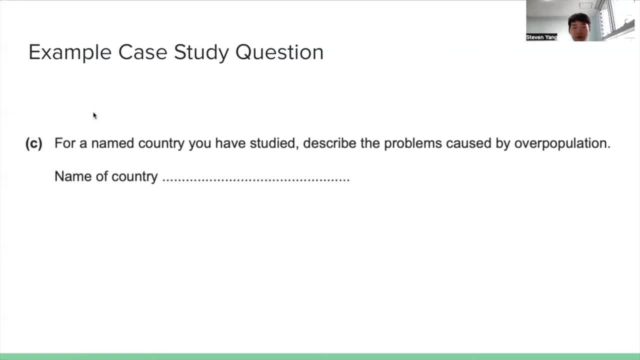 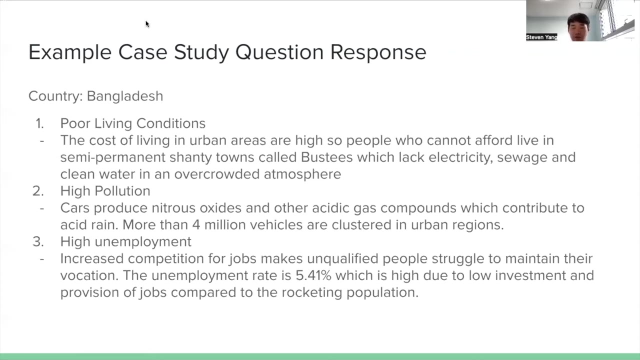 the problems caused by overpopulation, and i would like to advise you to pause the video and brainstorm three develop points with play specific detail. so now i hope you uh brainstormed your three points and i will show you my example of the response. so this is my brainstorming. so i chose, of course, bangladesh, which was my case study. 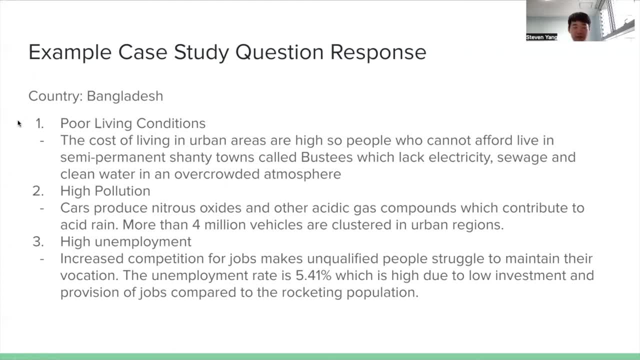 and this is my outline. so my first point is that the living conditions are poor, so the cost of living in urban area is high. so people who cannot afford, they live in semi-permanent shanty towns called busties, which lack electricity, sewage and clean water and they can't afford to live in. 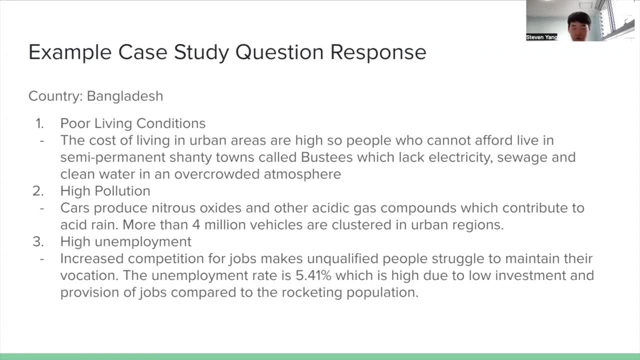 condos, so people can't afford to do that as well, for example, which is pretty decent. so the reason i chose this for is because it allows people to be at home when they don't have much in their families, and the other reason why i chose this is because it enables 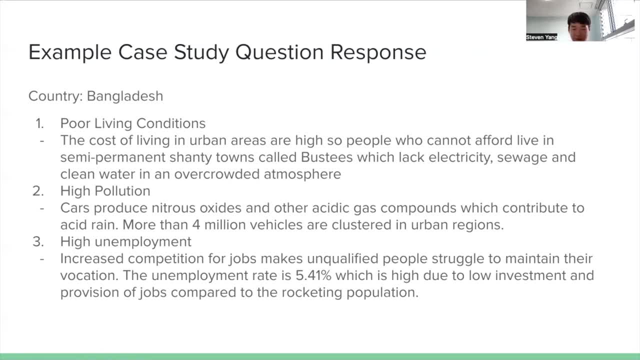 people to learn about the environment. it's also important to think of how you can protect yourself in this place, which is also important in our home, and i would like to point out that it removes all the stress from your environment. it removes all the stress from your kids and 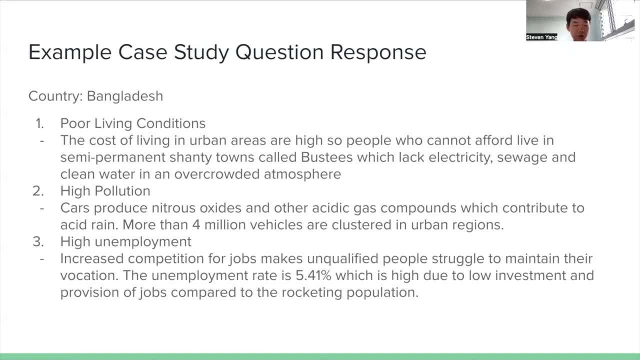 struggle to maintain their vocation. So the unemployment rate is 5.41 percent, which is very high due to the low investment and provision of jobs compared to the rocketing population. So you all can devise your responses in three paragraphs, one for each point, with